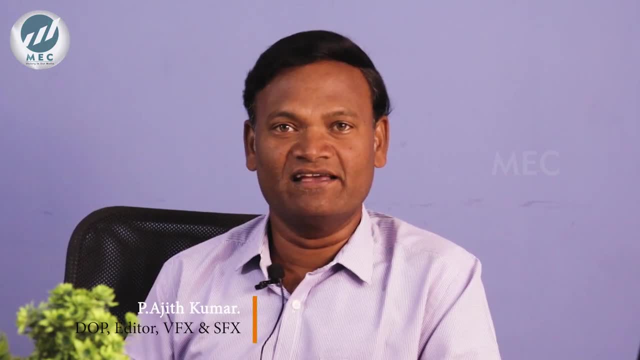 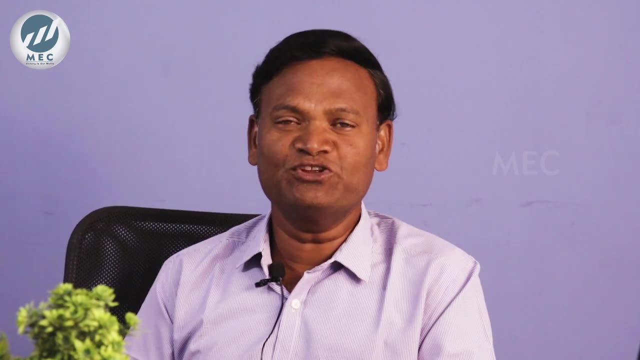 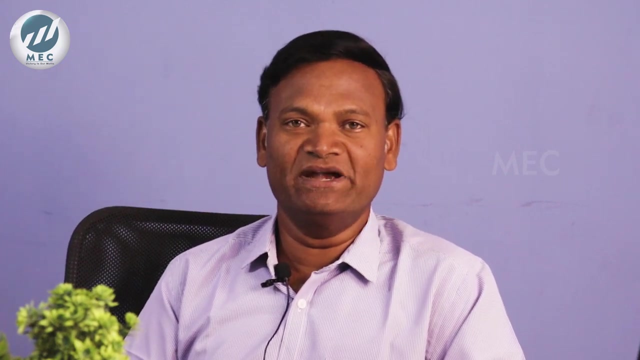 in our day to day life we are facing the challenges like the fasteners selection, as well as the fasteners where we can utilize it. First of all, we should see what is meant by fasteners. So fasteners means it's like joining of two metals or two non-metals. 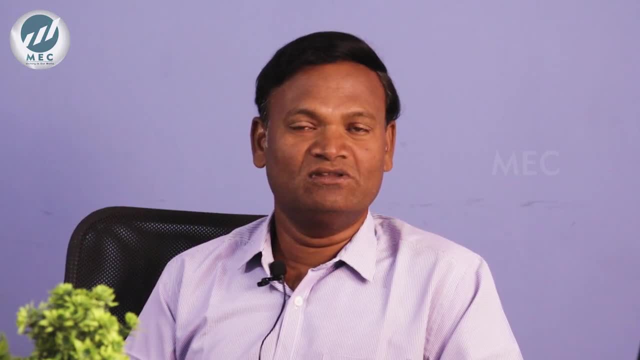 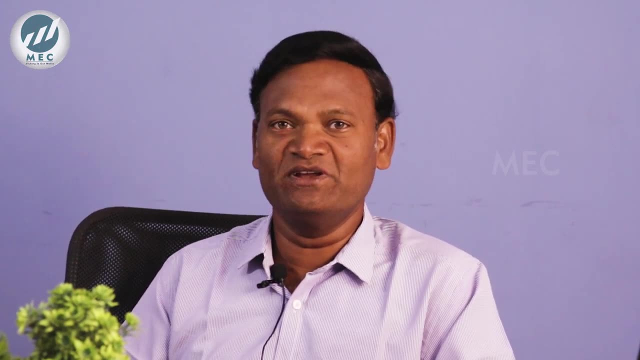 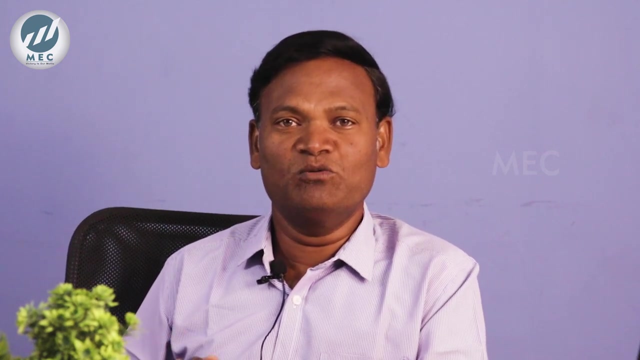 It may be anything right. So the joining process may be the permanent joint or sometimes it's temporary joints. So permanent joint means like welding and rivets, So once if it is welded we cannot remove that right. And one more is the temporary joints. It's like by using the bolt. 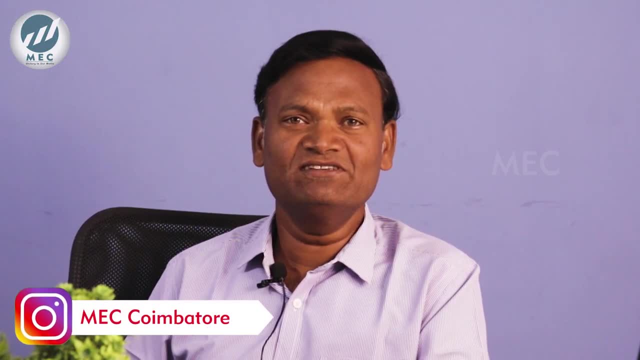 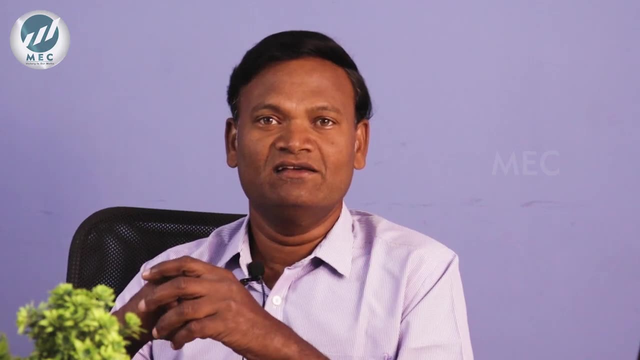 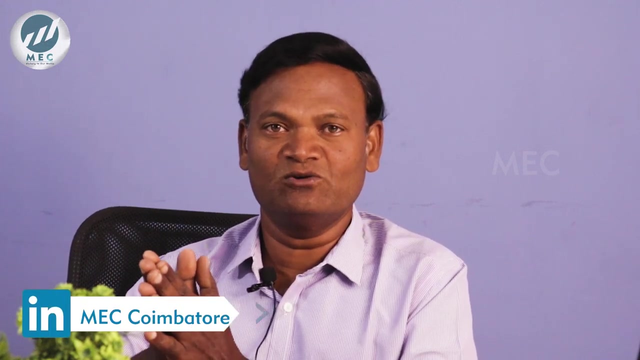 nut and washers. Even sometimes, if you have the like tie rod or something like that, we can hold that component. I just wanted to take a simple example like mounting bracket. So I wanted to take the mounting bracket and mount in the wall or any. 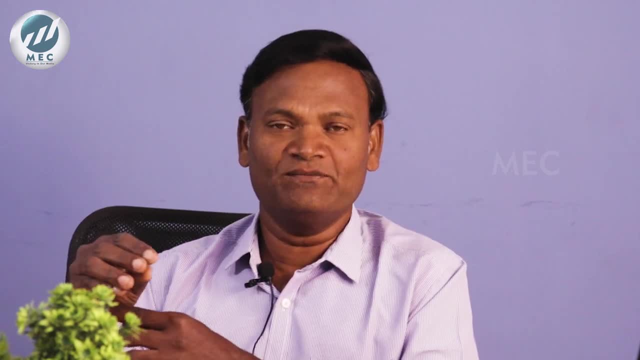 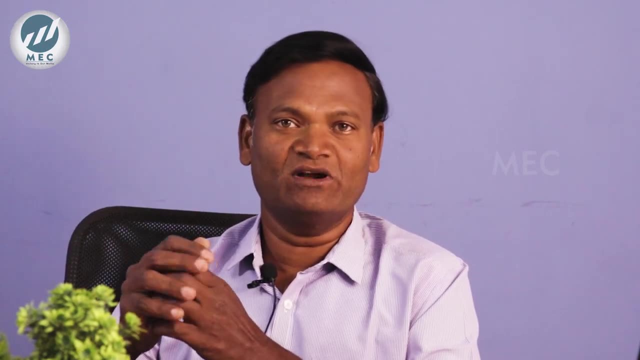 supporting structures, So by using the fasteners like bolt, washer and nut. So what type of bolt I can select and what type of nut I have to select? What is the basic parameter of this bolt and nut? So that's very important. 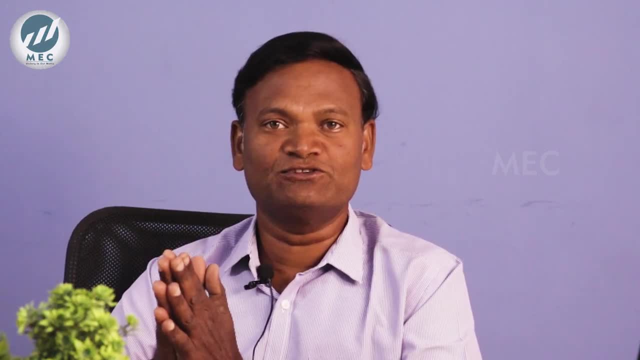 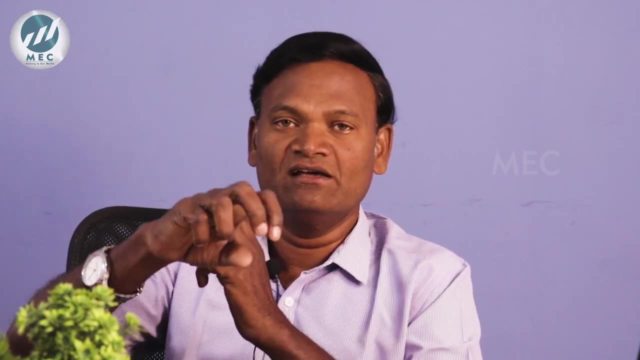 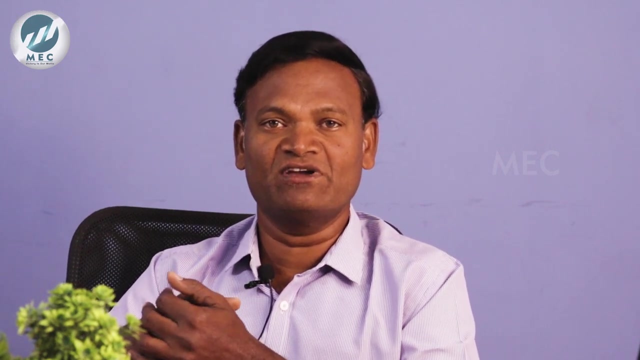 So mainly the bolt and nut selection which is based on what type of load is acting on the structure and what is the force which is acting on the where we are going to hold the bracket structure. So, once the load is acting on the particular structure, we have to select based 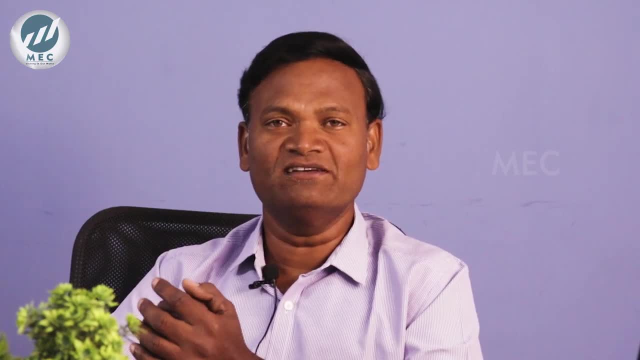 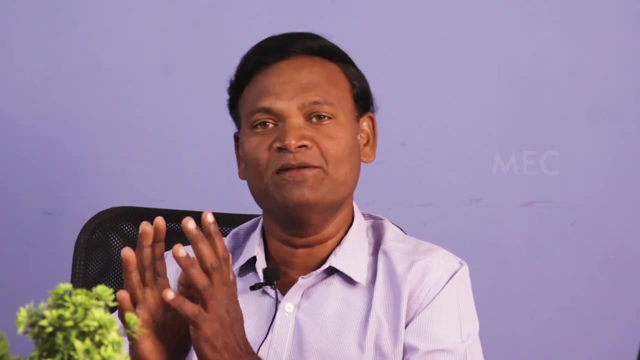 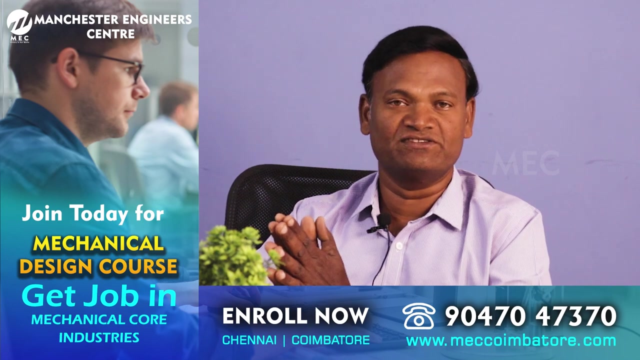 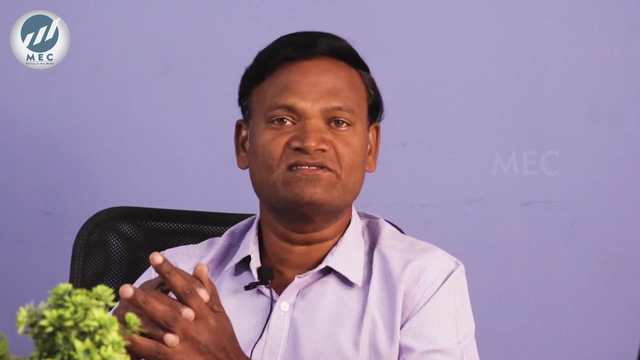 on that load Number one. Then the next part is the material selection. Even though if it is a fastener, there is a material. The material should be in higher temperature climatic condition and lower temperature climatic condition, Both wise And some places, even though some critical situations, like if you have a fuel tank or 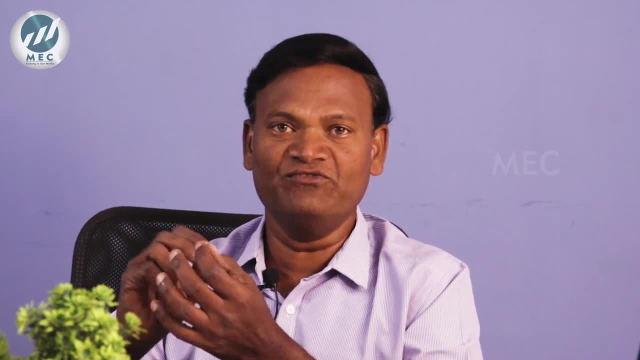 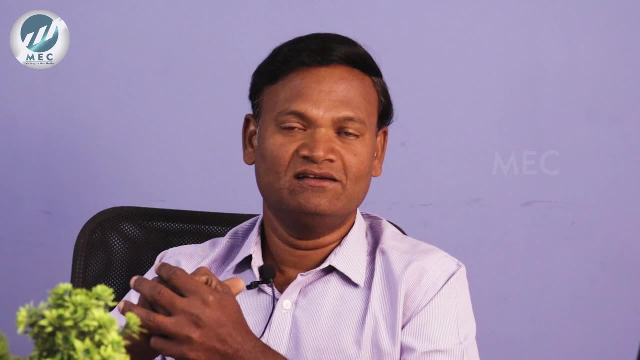 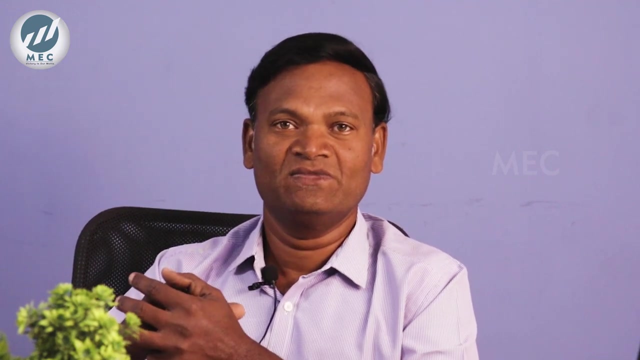 hydraulic tank. If you want to mount some bracket structure with the hole by using that hole, we have to mount the bolt and nut, Correct. It should not be leakage. So for that reason they are using like gaskets, Something like that. Okay, So how we have to select on this? Basically say, for example: 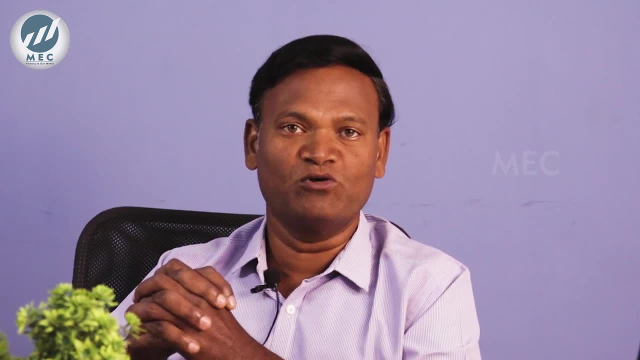 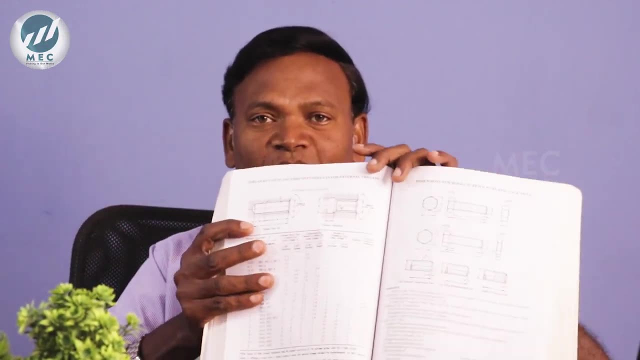 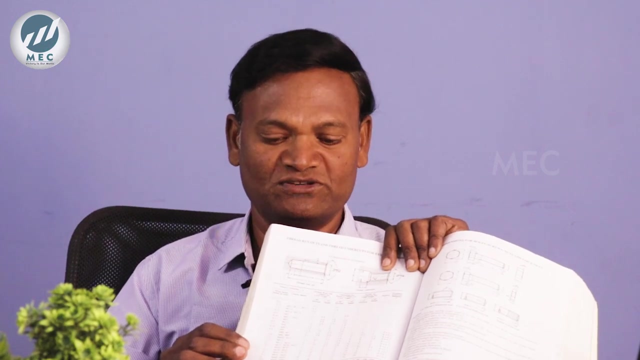 if you take the M8 bolt or M6 bolt. So the bolt selections it is mainly you have the data book. In this data book it is mentioned especially in the chapter 5. We have the selection of standards and selection of components. You just see that these are all the 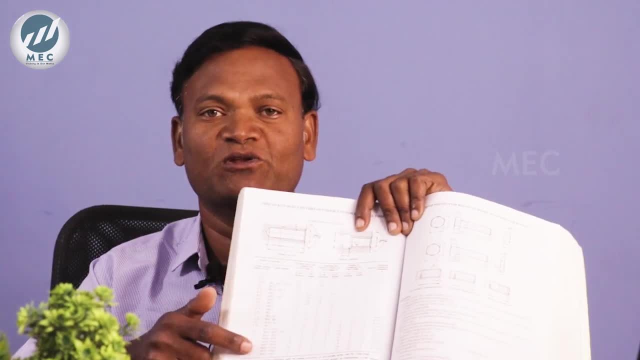 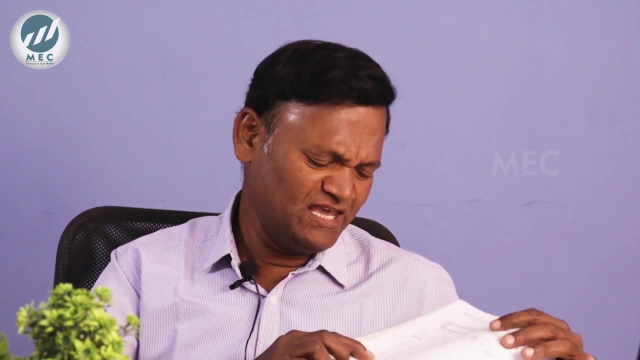 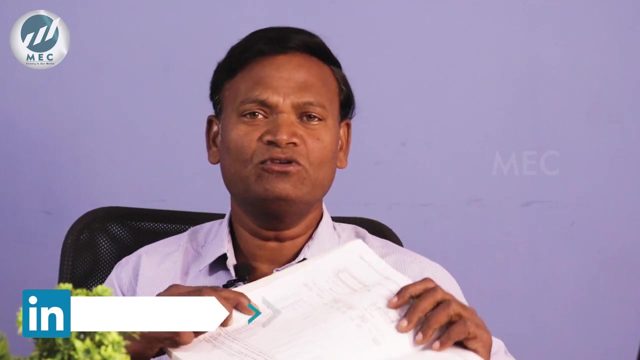 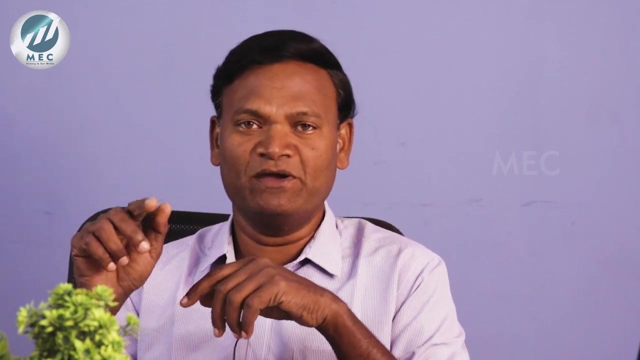 many type of bolt which is available in this particular page. Suppose say, for example, if you take M8 bolt, So this M8 bolt nearby there is the one more parameter, one more values is called pitch 1.25.. Always you should mention in this particular bolt, parameter like M8 multiplied by. 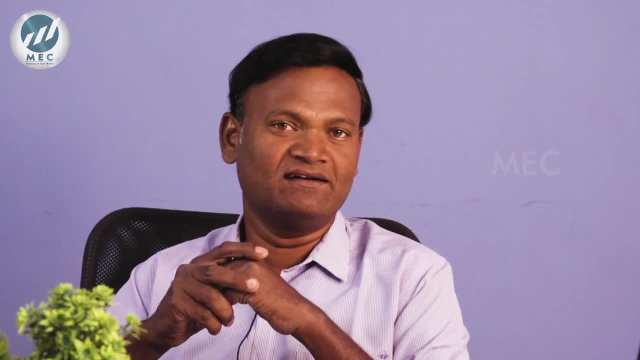 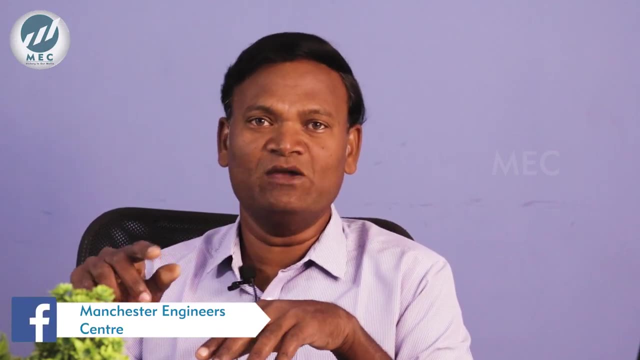 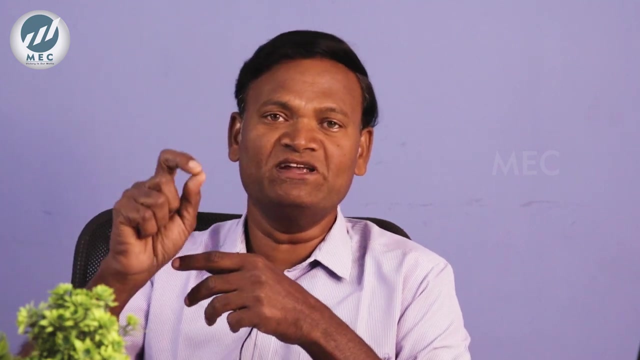 1.25.. So here M8 means metric thread. I mean M it represents metric basic diameter of 8 mm multiplied by 1.25 is a pitch Correct. So any drawing if he wants to take, especially in the fastness drawing, it should be mentioned like: 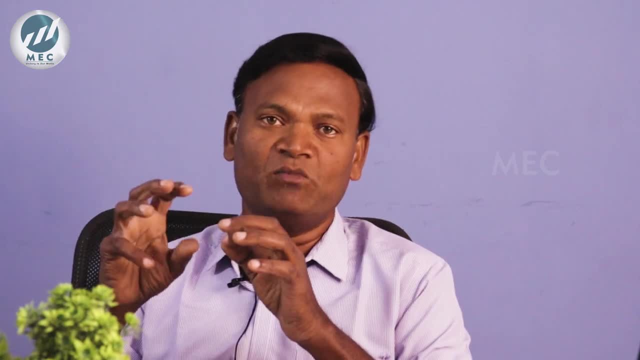 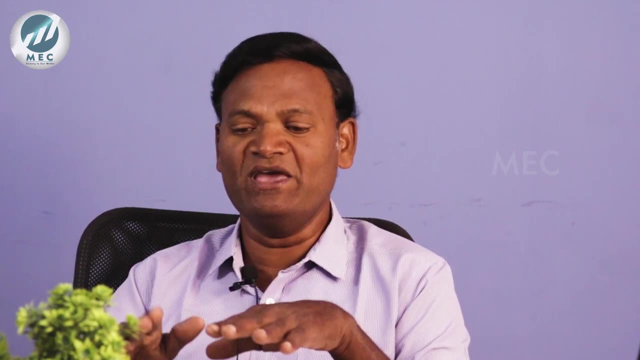 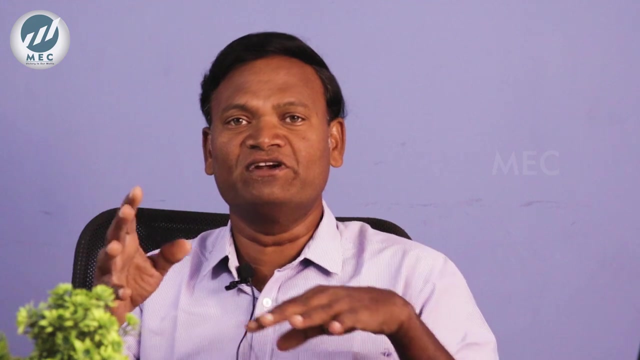 M8 into 1.25.. Which mean that by using this M8 bolt we have to hold that particular bracket structure Correct. So that is a basic idea about selection of bolt. Corresponding to that the type of bolt, suppose. if it is not with standing under particular load application, we have to replace. 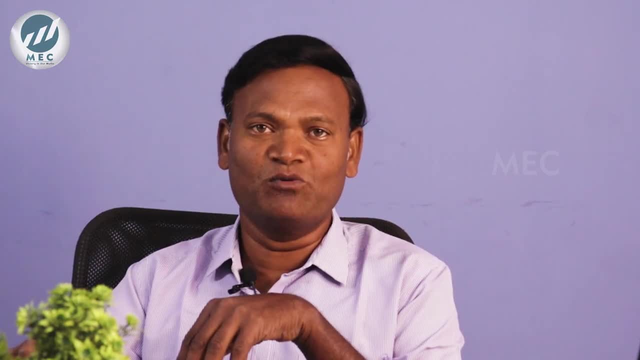 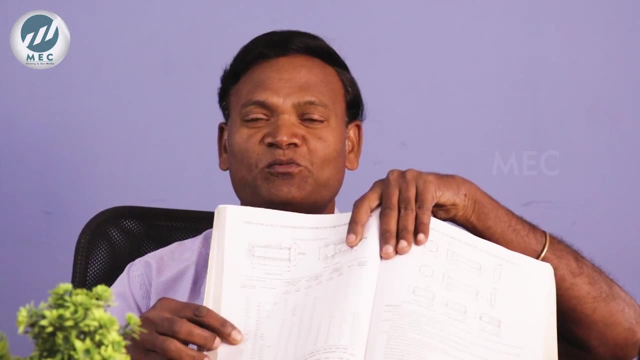 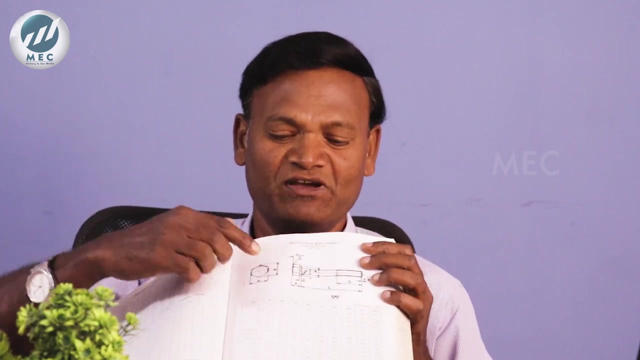 instead of M8 bolt, we can change it to M10 bolt. Even if you select this M10 bolt, then that bolt we have that pitches around 1.5.. So once if it is selected that, then here you can see that, whatever the type of bolt we have selected and this corresponding all the parameters, which is located. 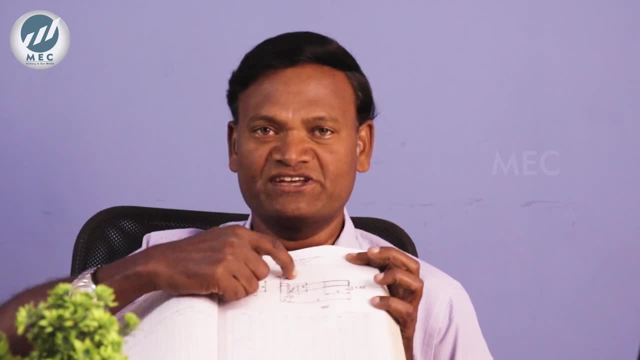 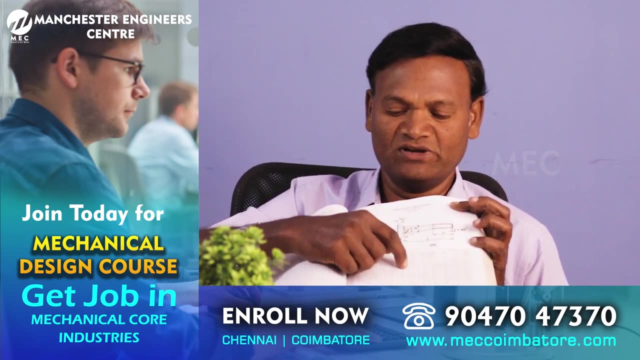 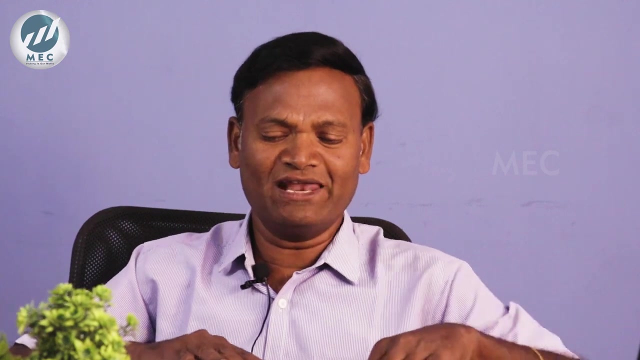 here. If you want to do the 3D modeling of this particular bolt section, you can take this particular standard values. this is completely as per ASME standard. So take this- all the values- and create this particular bolt. If you want to create a model like that, Then once if you selected the bolt, 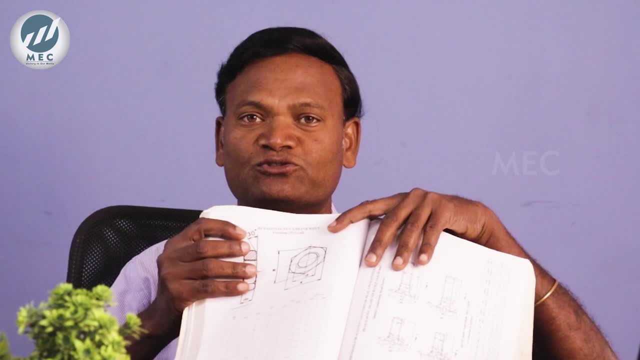 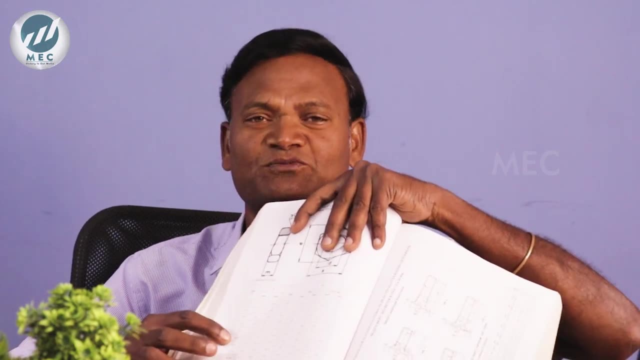 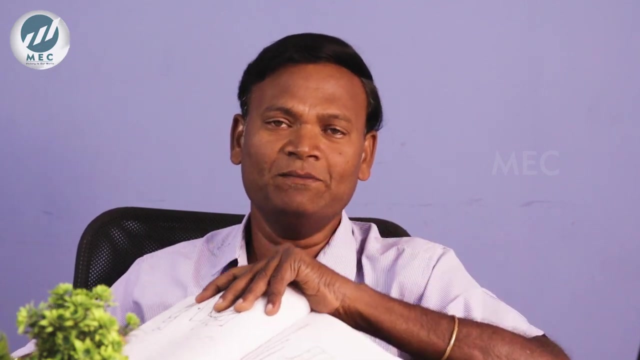 section. then automatically we need to select the nut. also, You can see here, whatever the bolt selected, the basic die of 10 mm, then corresponding, Not the parameters, everything which is available in this dinner jet have. So, by using the type of load, what they had to consider.